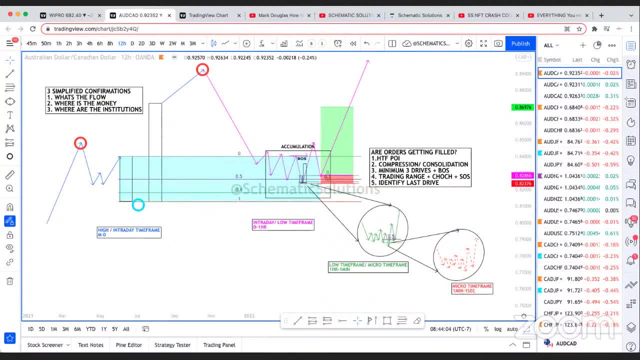 of our trading that we use every single day and just ultimately utilizing multiple timeframes in confluence with each other. So let's dive into it First things first. we have, plus or minus, about three to seven or eight confirmations In all reality, this list. 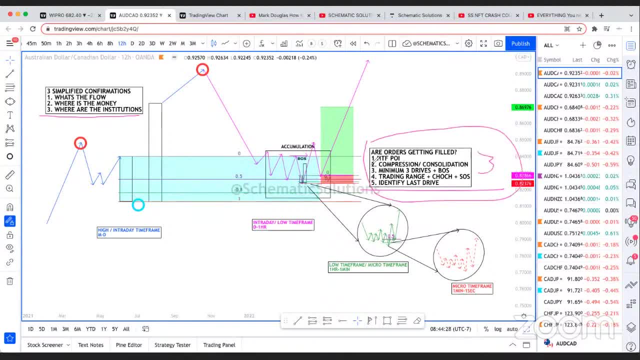 is typically around three confirmations itself. I usually just use higher time frame, POI, compression, consolidation, minimum of three drives, break of structure. So in all reality this is typically like a six-step confirmation. I did add a couple extra things just to. 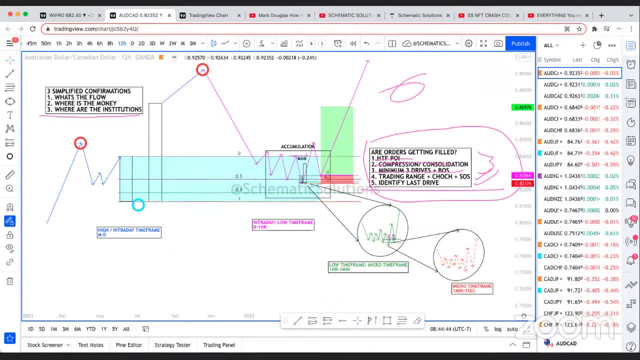 make it a little easier for some of the beginners to really understand these concepts. But yeah, if you already understand these concepts, you understand how to identify a schematic and all of that stuff. But first things first is what's the flow? What do I mean by what? 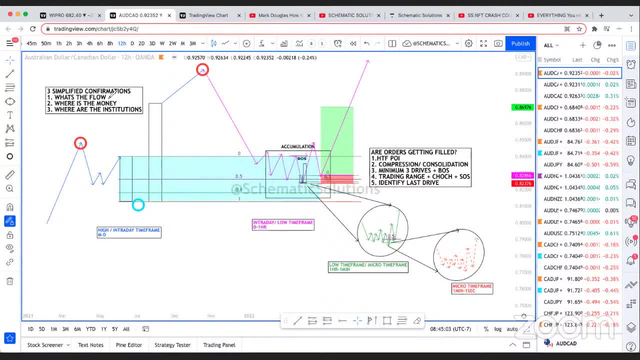 is the flow. Ultimately, we're talking about what is the flow of the market, what is not the order flow, but what is the structure. Now we can be talking about order flow when we're talking about this. Just keep in mind. 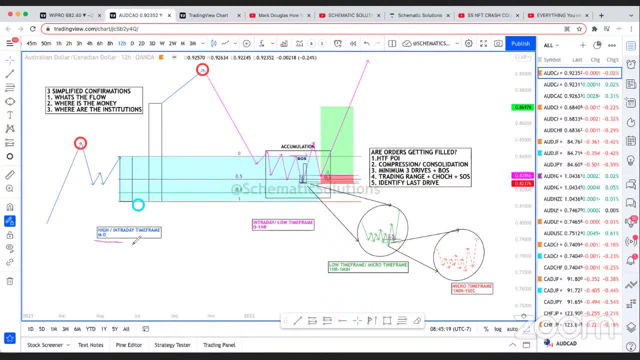 order flow is a lesser probability. So ideally we're going to want to start off either higher time frame or intraday. So let's say this is our higher time frame. For that higher time frame we're going to want to identify our current high or our current low first. So let's say we are 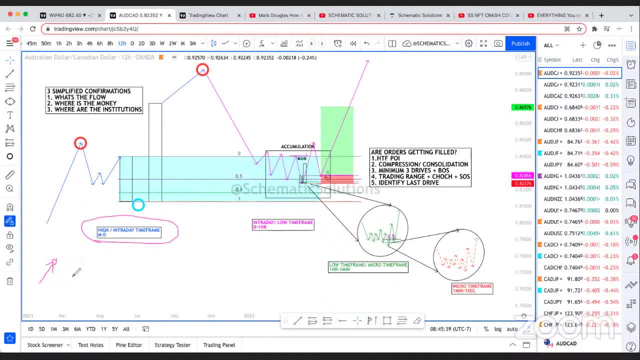 bullish, We're going to want to identify that current high. If we are bearish, we're going to identify that current low Make sense. So, since we're bullish, we could see we are definitely in an uptrend. We have our current high right here, Perfect, perfect. Then we want to ask ourselves: 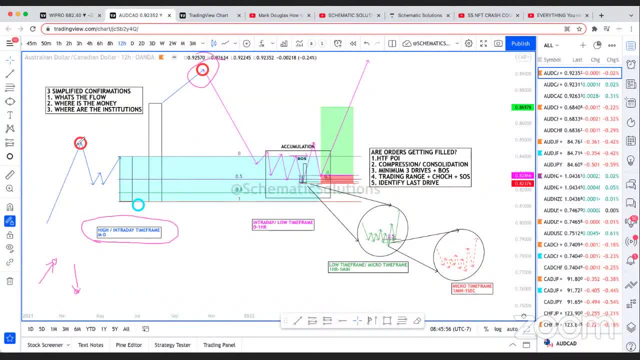 what is the high before this current high? Can we agree? this is the high before it. It's not this high, because this high was not higher than this high. Perfect. So this is the high before it, which means this is our low. 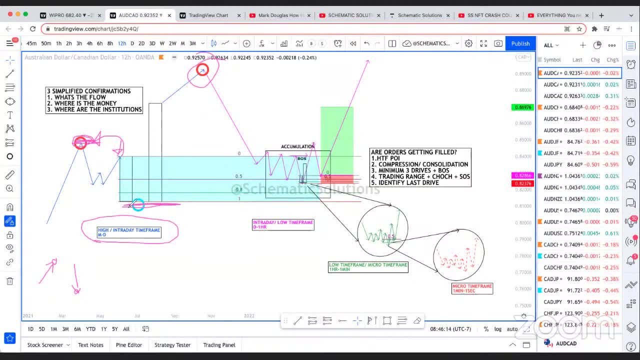 Now, keep in mind, I'm not talking about bodies, wicks. We use wicks as structure, And if you're wondering why, it's a whole other video- But ultimately, inside of that wick is a candle right, Exactly So. we don't use candle bodies as structure, We're talking about the. 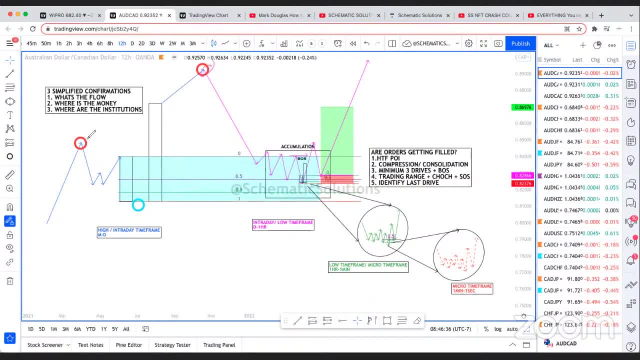 actual wicks, in case that was your question. Now, high, high, low, maintaining we have our structure. It's extremely simple. Step number two: we want to ask ourselves: where is the money? When we're talking about money, we're simply talking about liquidity, And you can use. 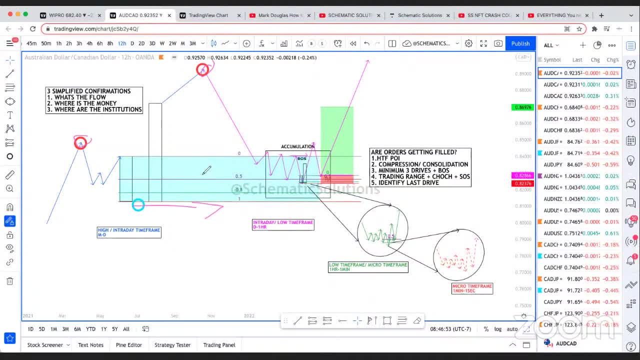 liquidity to bring you back towards your entry. But to be extremely basic, we're only going to use liquidity for a target. So what is liquidity? Equal highs, equal lows, trend lines, opinions in the market, obviously. And then we want to ask ourselves: where is the money? And if we're, 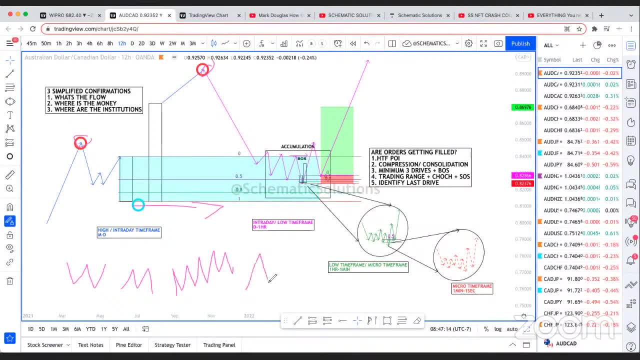 and last but not least, every single high and every single low holds liquidity. So let's say, there's no equal highs, no equal lows over here, but we have a single high right here. Can we agree? this is our liquidity, Exactly, And obviously we'll have lower liquidity points as 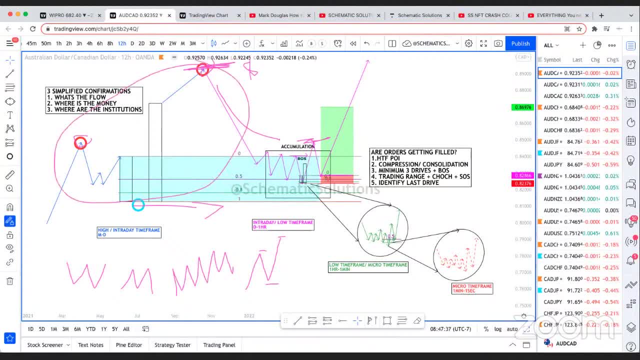 price comes down, But as of just the higher timeframe price action. this is our liquidity. So we have our structure And then we want to ask ourselves: where is the money? And if we're structure, we understand where our money's at Now. where are the institutions? And this is 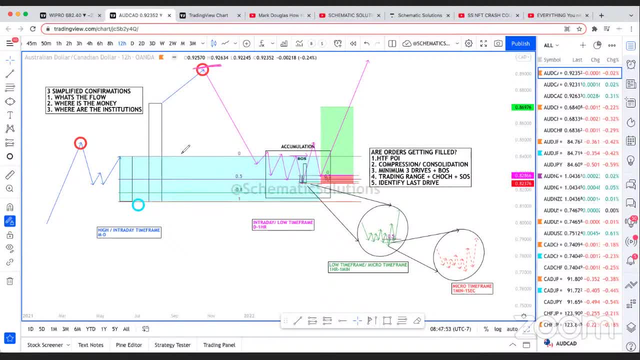 ultimately asking: where is the supply and demand, Where are the POIs, Where are the OBs, the order blocks, whatever you call them? I personally just call them point of interest or schematics. Now, that's what we're looking for. We're looking for either that last push down. 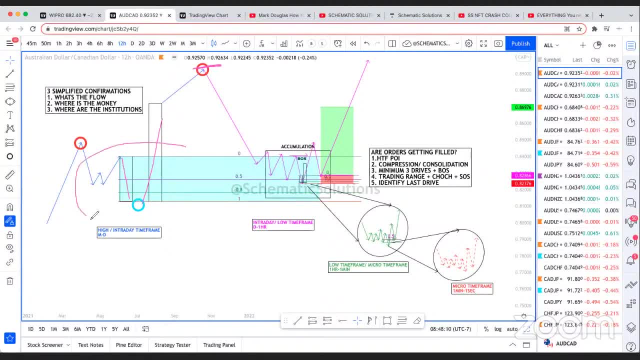 before the push up move, We're looking for our accumulations, our reaccumulations, whatever the case may be. So let's say this was our reaccumulation. If you trade Wyckoff, you understand that. Or let's just say this is. 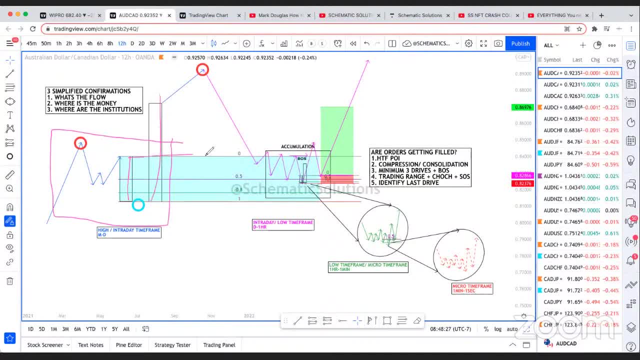 that last push down before the push up move. We're going to identify that point of interest, measure it out and we're looking for price to get into 50 and or 80%. Now here's the thing: If 80% is less than the 10 pip, stop loss. 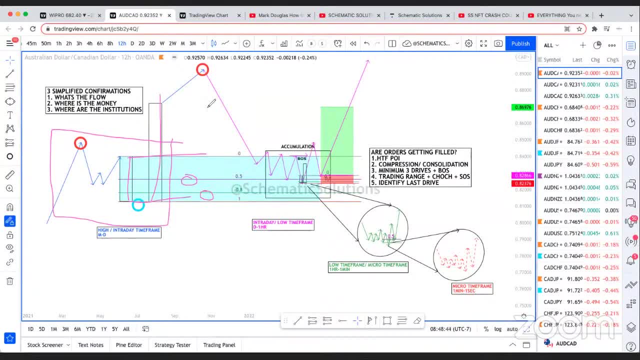 50% is less than the 10 pip stop loss and it's higher time frame structure. I'm willing to place some risk on it Now. it's going to be very rare that you identify a large move in the higher time frame and it's going to be less than a 10 pip stop loss. So in that case, 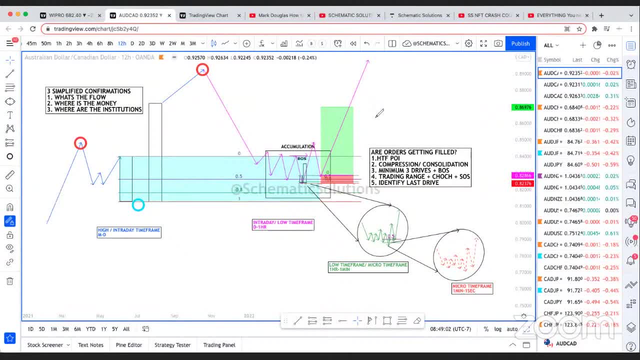 scenario, what you're going to have to do is wait for a schematic. So what we're going to ask ourselves is: are orders getting filled As price comes into the area we're expecting institutions to move price away from? are they filling orders there? So what are the 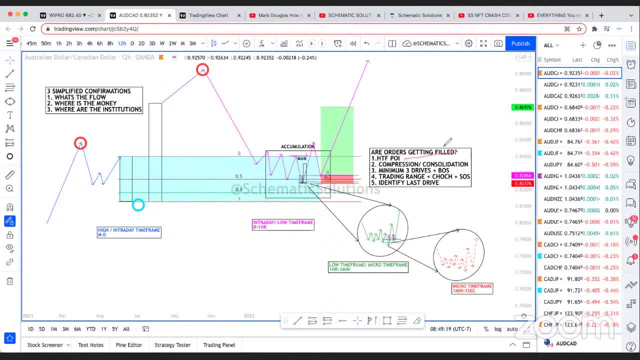 confirmations of this. First things first. we want to be in or near a higher time frame, point of interest. Step number two: we want to ask ourselves: okay, are we compressing or are we consolidating? Compressing, I would say, is price getting close together Instead of just falling. 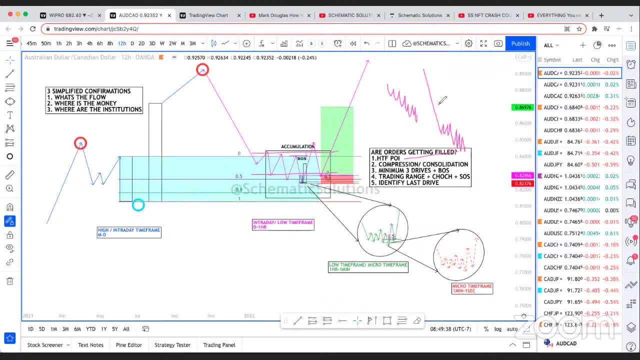 it's price literally starting to just move closer together and consolidation: Is price actually going sideways. Then we want to ask ourselves: do we have a minimum of three drives and our break of structure? I emphasize on minimum of three drives because we can have. 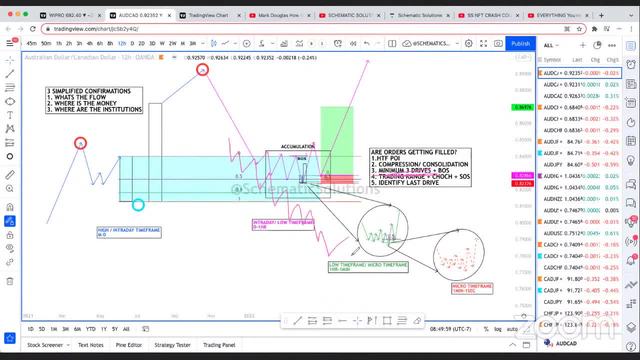 26 drives: One, two, three, four, five, six, seven, eight, nine, 10, and our break, Once we get that break. this is our schematic. This is our schematic. So, minimum of three drives. 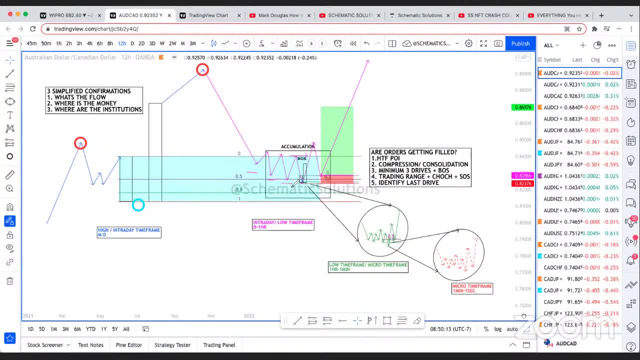 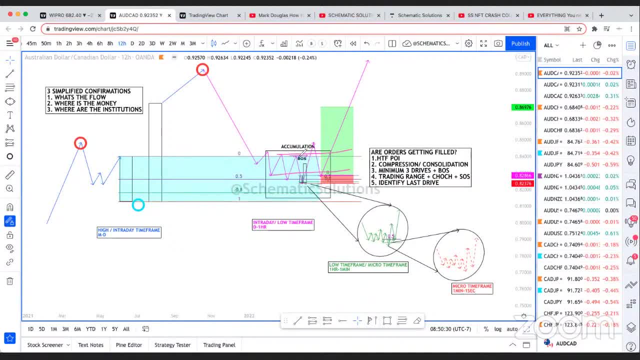 which is just going to be where price identify or where price spends the most time going back and forth. Two: our trading range is going to be our climax to our AR. If you don't know what that is, check out one of the in-depth Wyckoff videos. 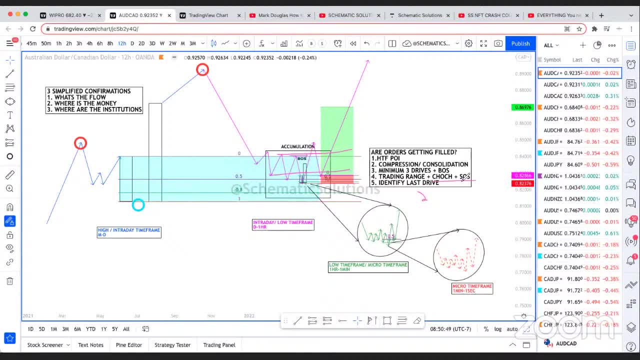 Three. we then want to identify that change of character And our change of character. once again, it's going to be our trading range climax to AR, but how do we know something's our change of character. So it's ultimately going to be that. 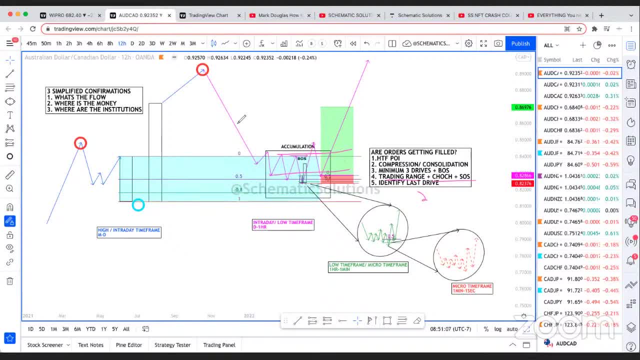 first, deepest retracement relative to the last couple. So if we could see, this was our high, this was our high, or sorry, this was our high, this was our low. and then price retrace. Okay, how deep did that retrace? Not too deep, But now we have. 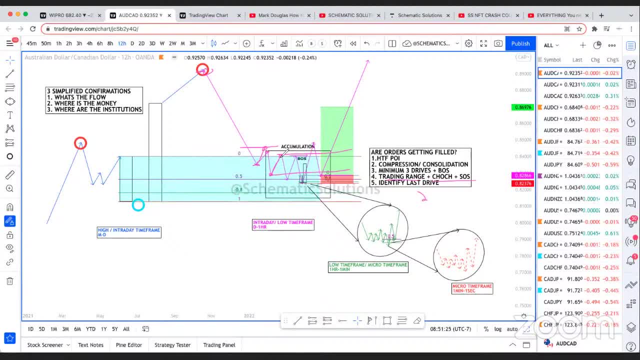 this is our high, this is our low. How deep did price retrace? Price almost retraced, 100%, right. So that's that first deepest retracement right there, giving us that change of character. Now our next event that we're. 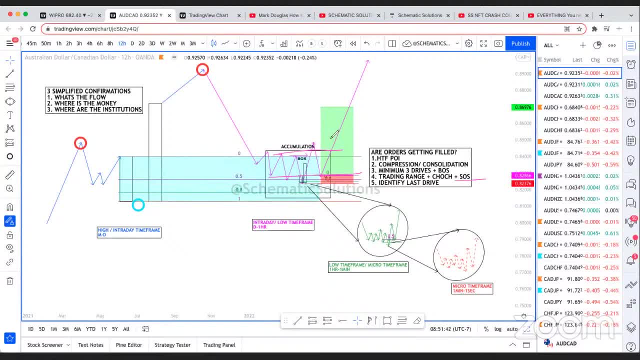 we're going to want to identify is going to be the sign of strength, which is going to be price breaking, structure and exiting our trading range. Once we've identified that, we can identify our last drive, measure out 50 and or 80%. 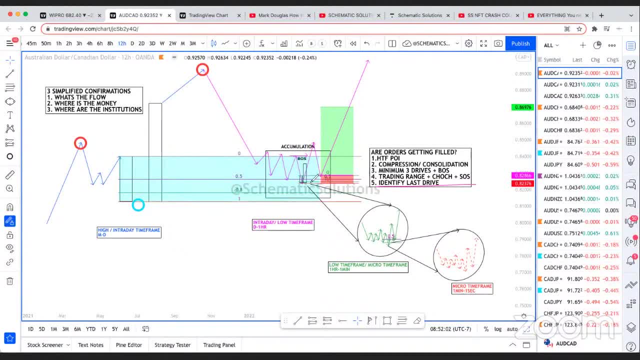 and take our limits if, and only if, it's worth it. Now, let's say, since this, since we were looking at the price, we're looking at the higher timeframe here, and this is the intraday timeframe here, let's say it's not worth it. So, as price, 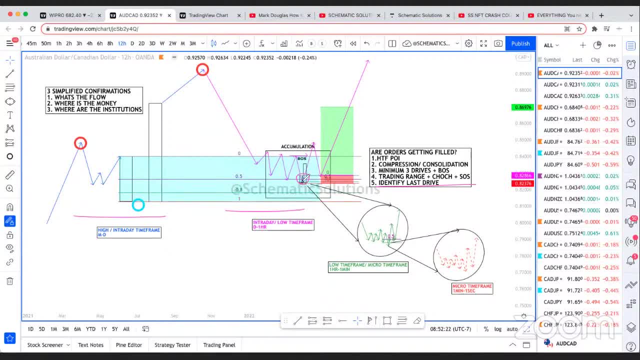 was down inside of our spring. we scaled down to the lower timeframe from the intraday and we saw this price action. We are in, or near that higher timeframe POI: yep, We have compression consolidation. We have our minimum of three drives and our break of structure: yep, okay, perfect. 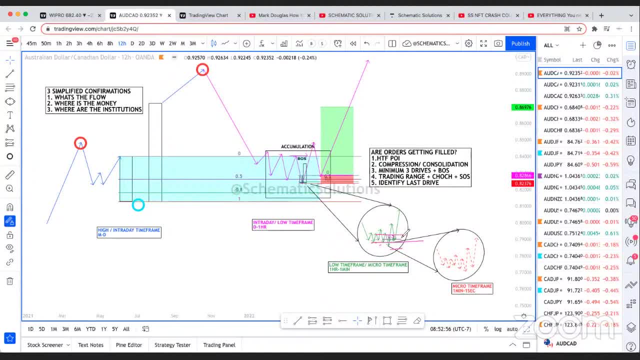 Where's our trading range? So looks like price spins the most time there. It's also that first deepest retracement relative to the last one. Where's change of character? Obviously, we just knocked that out. Where's our sign of strength? 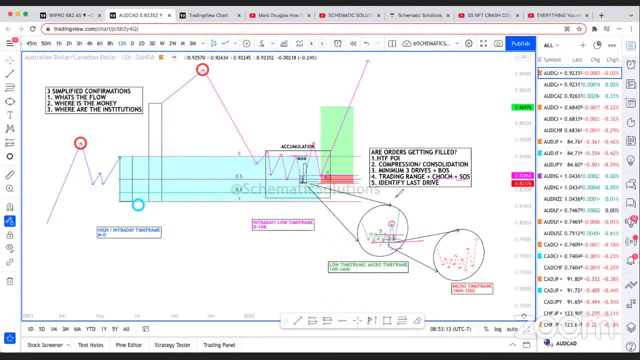 Sign of strength, the break of structure and exit of our trading range. Identify the last drive there to there. If it's worth it, place your entries 50 and 80%, splitting our risk. So this could be a lower timeframe through a micro timeframe. 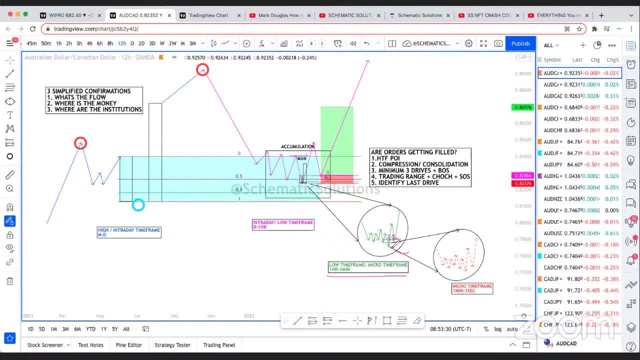 But now let's say we were able to see inside of this spring and scale to an even smaller timeframe- inside of the micro timeframe is the one minute through the one second- and caught this schematic. are we in that higher time frame? yes, we have compressed consolidation. yes, do we have a minimum of three drives in our 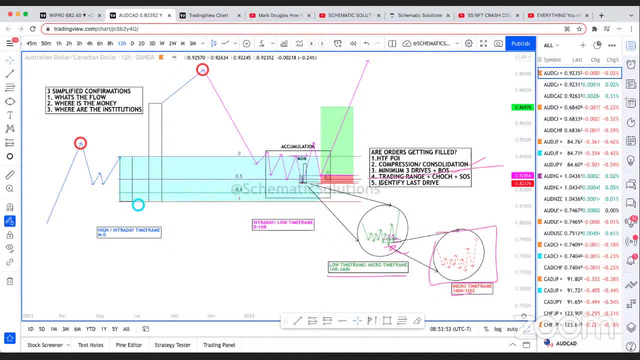 breakup structure. yes, do we have our events? yes, we do. do we have that last drive boom, 50 and 80. take your trade and this entry is how we catch those one to 100s, one to 50s. um, in those large r to r trades, consistently it's due to one, the lower time frame, because keep in mind the lowest. 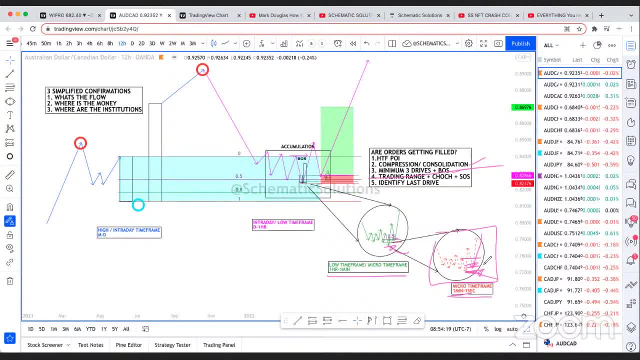 the lower the time frame, the lower the stop loss is going to be, which means the higher we go- or technically we don't have to go as high to catch that high r to r- but obviously the higher we go, um, the r to r is going to go crazy. obviously, obviously, obviously. but this is really how we. 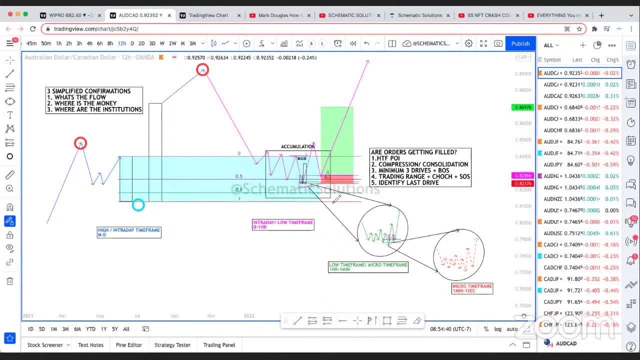 ensure to catch, or how you can turn a 1-20 trade into a 1-100.. Did you guys catch that? Literally everything that you're doing, if, let's say, you're catching consistent 1-20s, 1-30s. 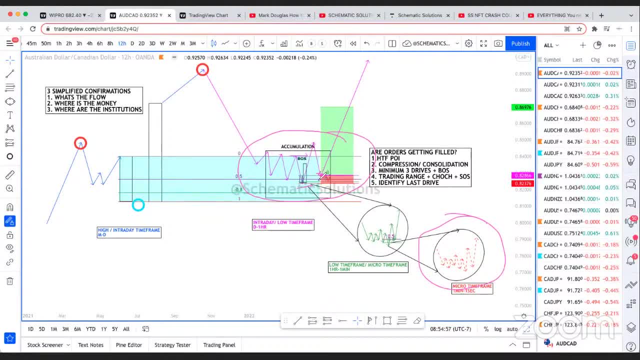 instead of catching those 1-20s, 1-30s, not instead of still catch those, but then try to dive into the spring and or the test and catch those fractal schematics out of the lower timeframe and or the micro timeframe. 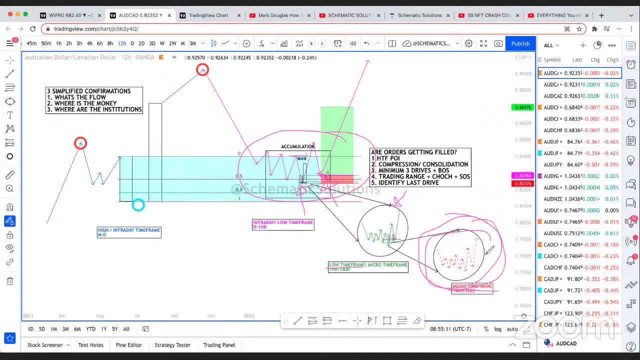 And the reason why I did the micro with dotted lines is because the micro timeframe is going to be relatively hard to see sometimes. So it's really something to where you're really going to have to train your eyes with. but this utilizing higher timeframe with the intraday timeframe,